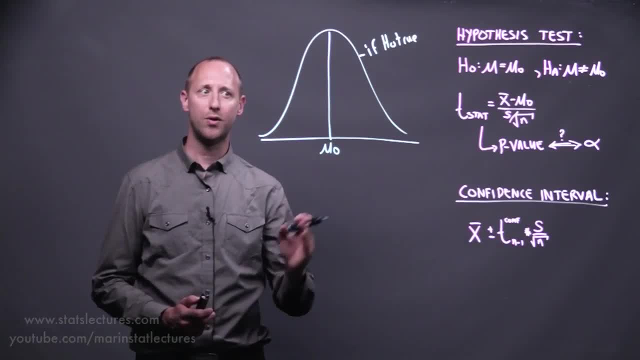 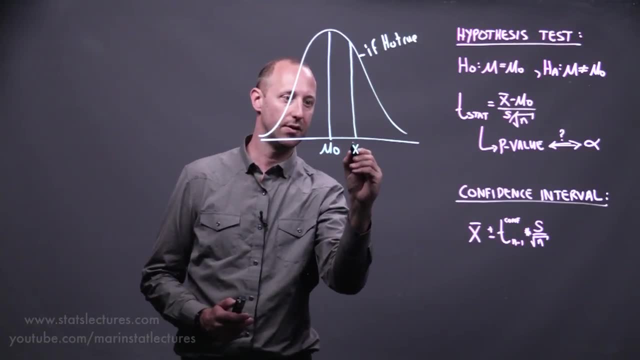 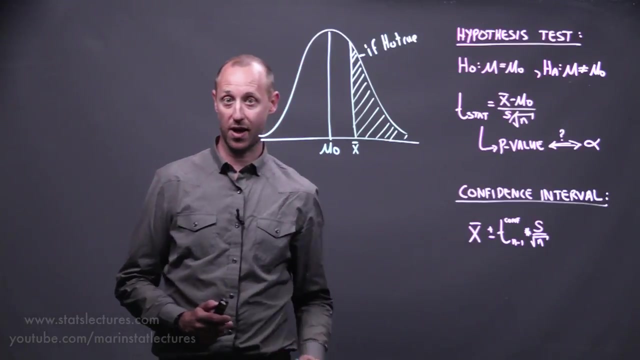 So here's what we expect the sample mean to be. We know it's going to vary a bit. Then we calculate some test statistic. Suppose that the sample mean we got was here. We're going to end up standardizing this or calculating a test statistic and a resulting p-value. 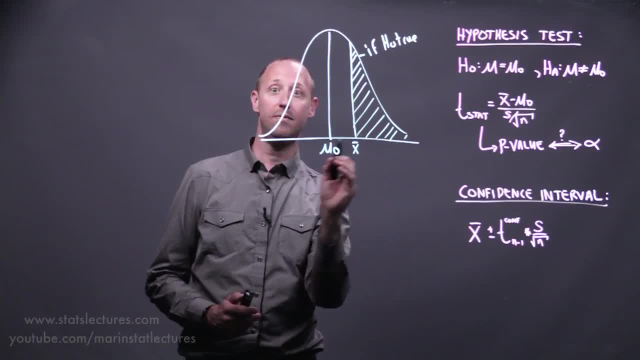 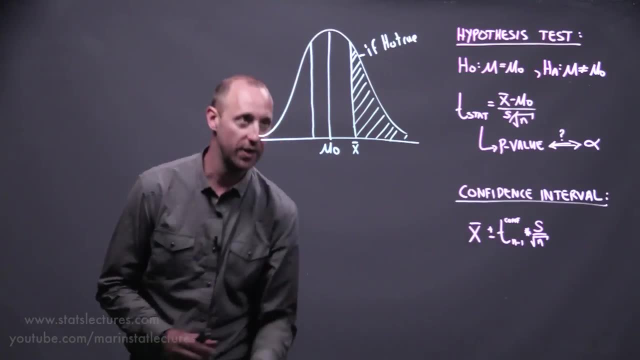 which is going to tell us how likely were we to get this estimate or one more extreme. Okay, in the case of doing the two-sided hypothesis test, we're looking at the question: how often will we see deviation This large in absolute value? 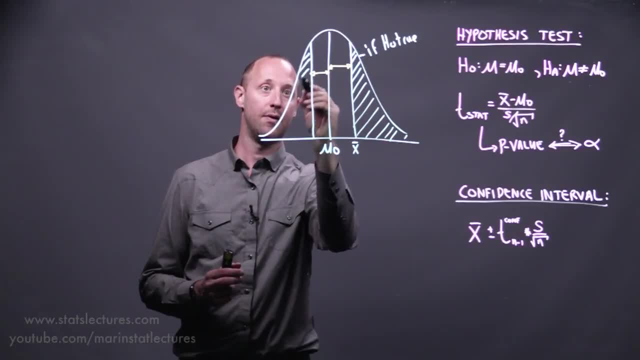 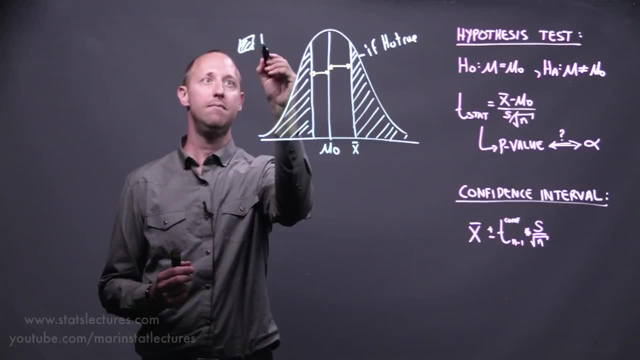 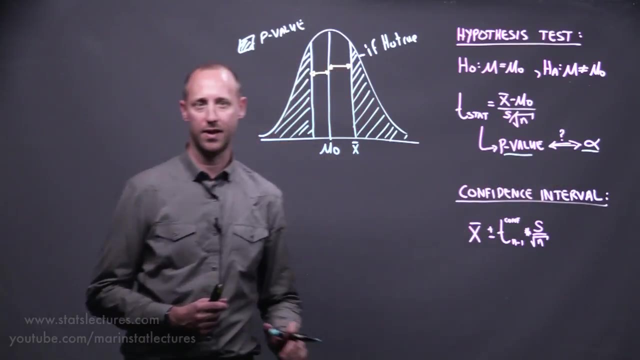 How often we get an estimate this far or further from the hypothesized mean. All right, so again, this shaded area here is what we call our p-value, and we compare that p-value to some alpha. If the p-value is larger than alpha, we fail to reject our null. If it's smaller than alpha, we reject our null. 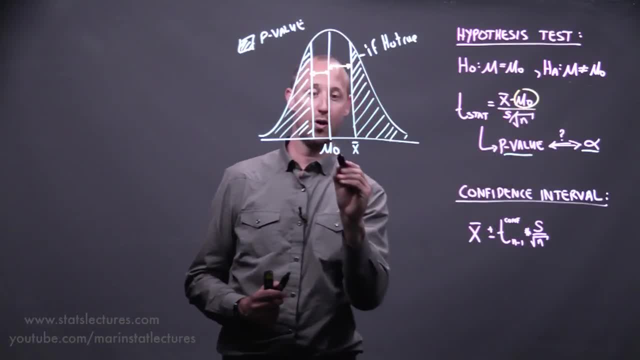 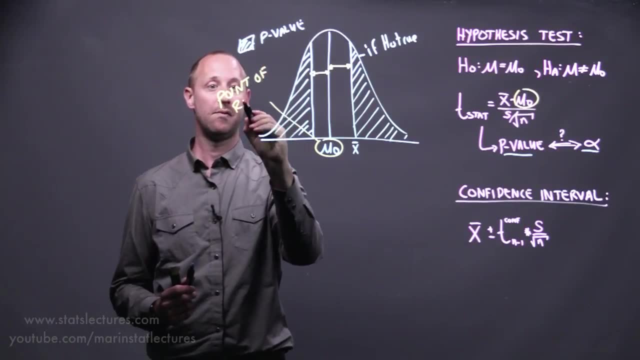 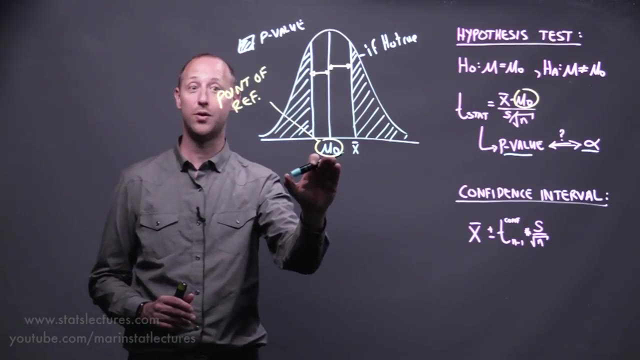 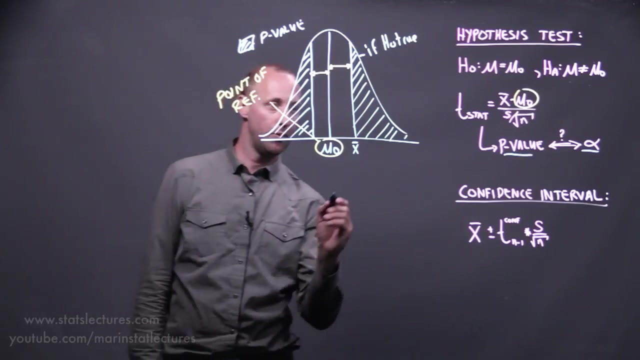 You can notice that in hypothesis testing, mu-naught- this here is our point of reference. So all the statements we're making are looking at how does our estimate compare to a null hypothesis, because that's our point of reference. When looking at a confidence interval, what we do is we go, so let's just extend these downward. 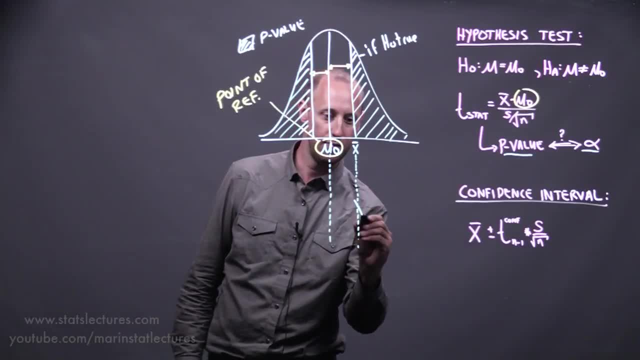 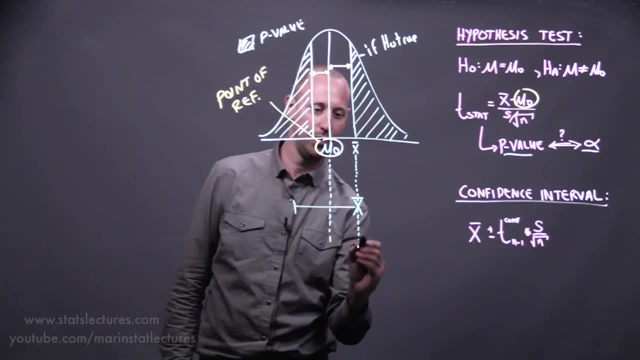 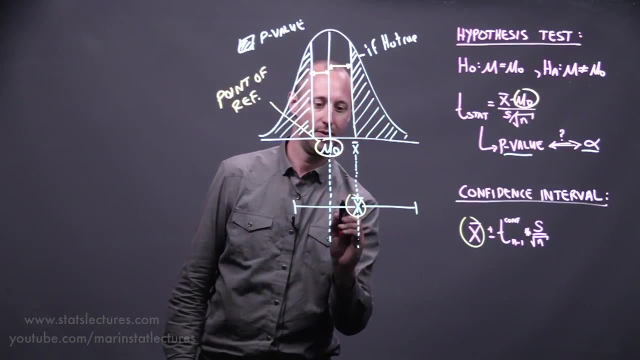 we go from our estimate and we tack on a margin of error Minus roughly two standard errors, plus roughly two standard errors. We can see here for confidence intervals, the sample estimate- here the sample mean- is our point of reference. 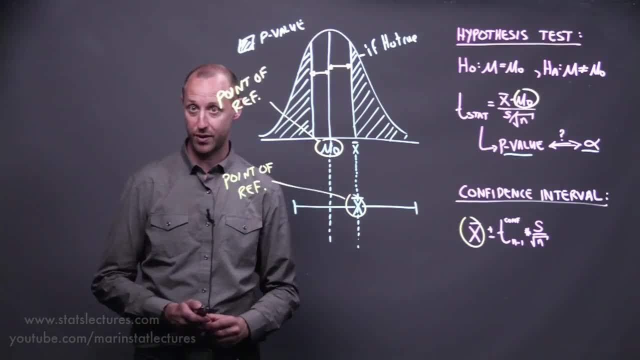 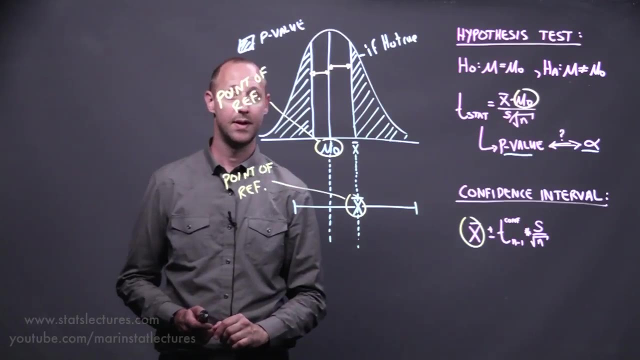 So if we want to use this- the confidence interval- as a hypothesis test, we can check: does the null value fall within that confidence interval? Okay, if the null hypothesized value falls within the confidence interval, then the p-value is always going to be larger than that alpha of five percent. 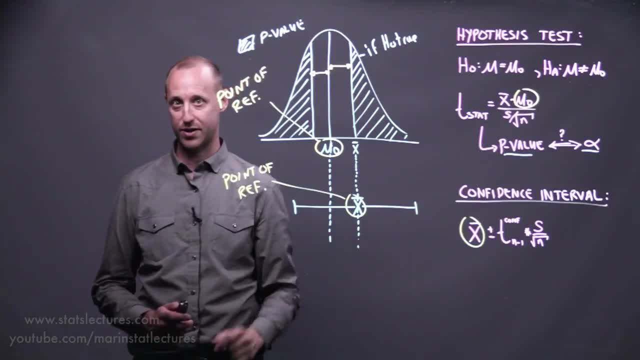 If the null hypothesized value was outside of the confidence interval, the p-value is going to end up being less than five percent. Okay, so the two of these- the test or the confidence interval- are always going to agree in the conclusion you reach.